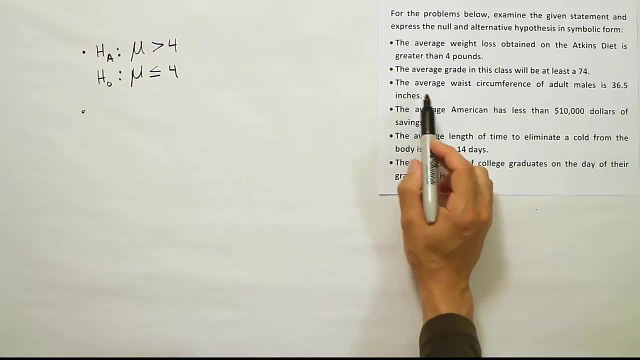 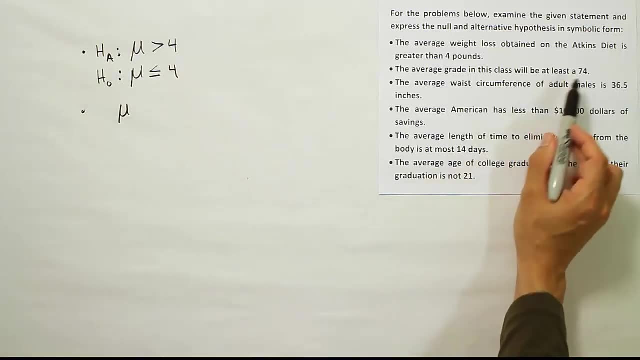 Okay, so that was the first one, Let's do the second one. The average grade in the class will be at least a 74. So we know it's about the average, And to say it's at least 74 means that it will be that or higher, right. 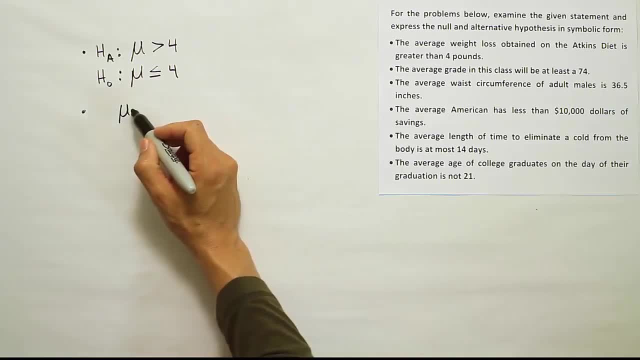 At least means the minimum. So it'll be 74 or higher. That means the mean will be greater than or equal to 74.. Now this would have to be HO, because this claim has an equal sign. That means our pair would be HA. 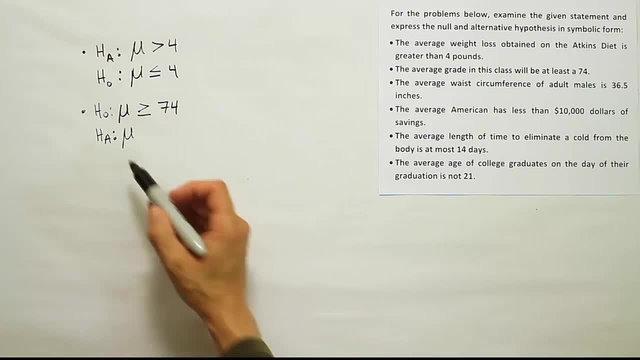 And this would be the complementary idea. So if you're not greater than or equal to 74,, the only way that's not true is if you are less than 74, right, It's the only scenario where this isn't true. The top one isn't true. 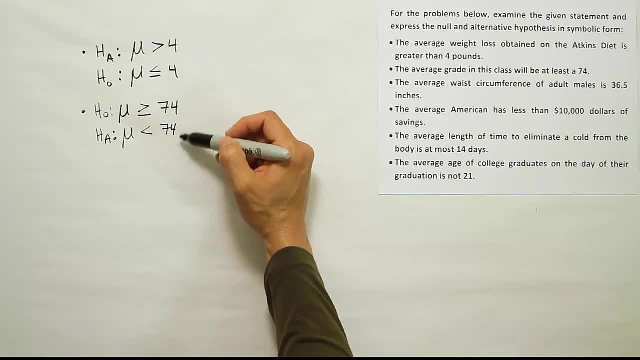 Only when the mean is less than 74. So these two together form all the possibilities. Okay, our next bullet. The average waist circumference of adults males is 36.5 inches. So again, this is a claim about the average right. 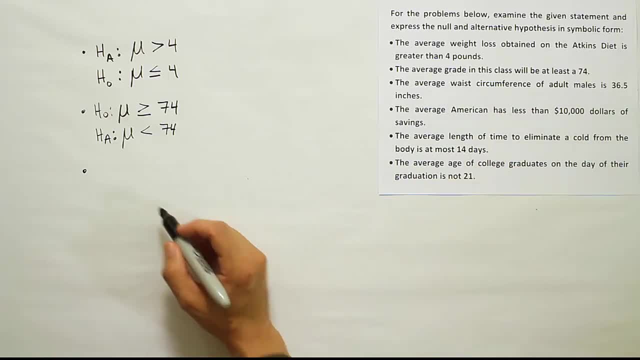 The average waist and circumference of males is 36.5.. The average is is, as an equal sign, 36.5.. Okay, and again, anything that has an equal sign in it is going to be HO, because it has an equal sign. 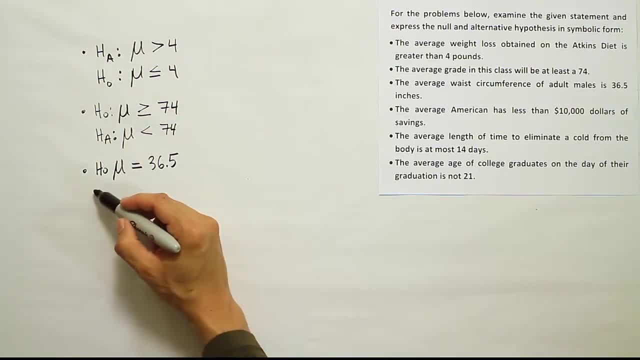 Right. Any one of these that has an equal, they're paired up with HO. The alternative hypothesis is going to therefore be a complement of that, And if you're not this, it must be not equal to 36.5, right. 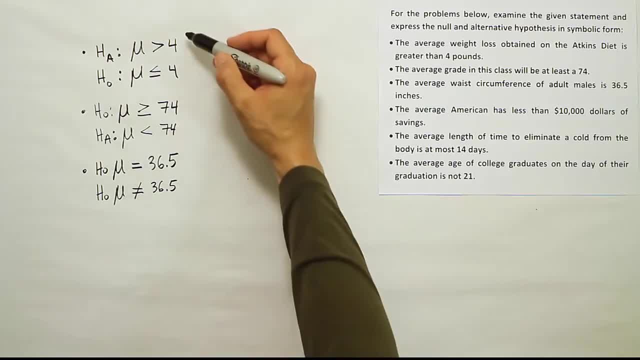 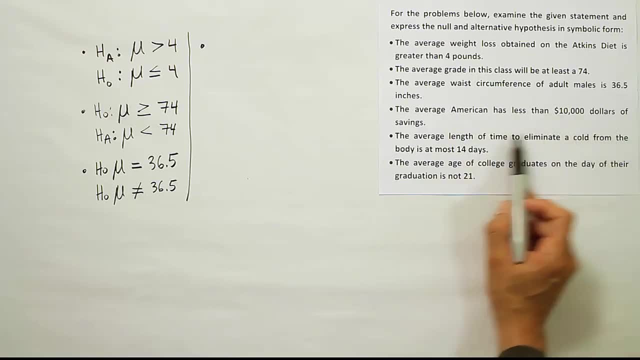 Okay, so that's the first three done. Let's do the next three right next door to these. Okay, the next bullet here, The average American has less than $10,000 of savings, So the average is less Less than $10,000. 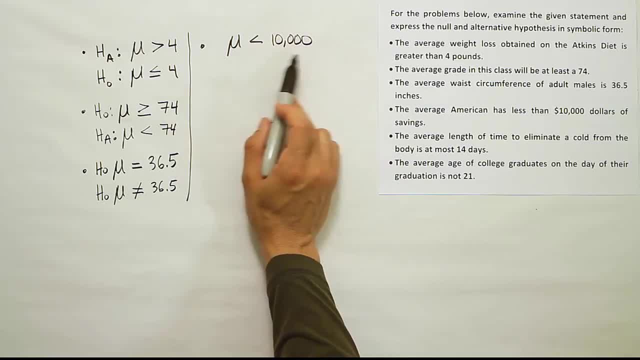 So the amount of money the average American has in the bank is, on average, less than $10,000.. Okay, Since this does not have an equal sign, since it's either less than, greater than or not equal to any of those three symbols, make it HA right. 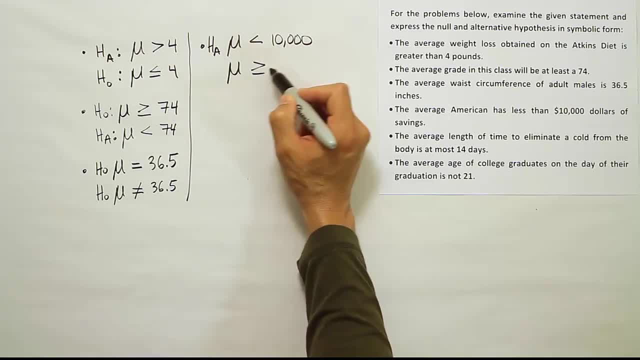 Now the opposite of that, then, is going to be greater than or equal to 10,000.. So that's the complement of the other scenarios. If you're not less than 10,000, it's greater than or equal to 10,000.